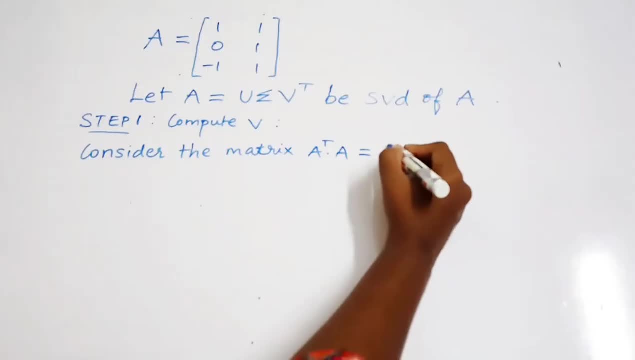 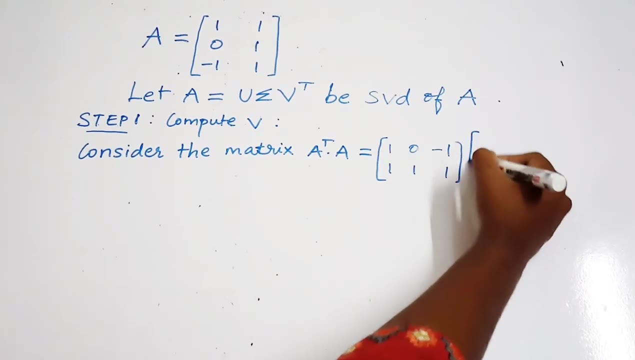 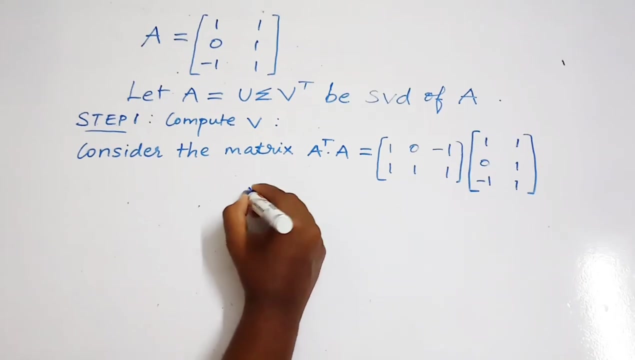 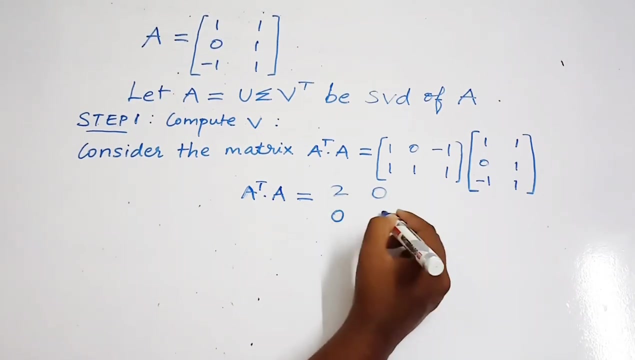 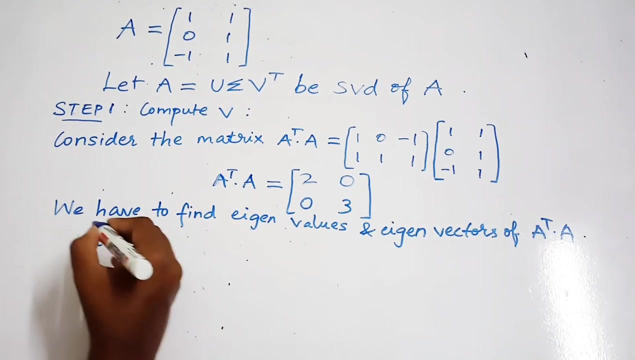 A. So we have to find the value of A transpose A. So now A transpose A is 2, 0, 0, 3.. Next we have to find eigenvalues and eigenvectors for the matrix A transpose A. So let lambda square minus S1 lambda. 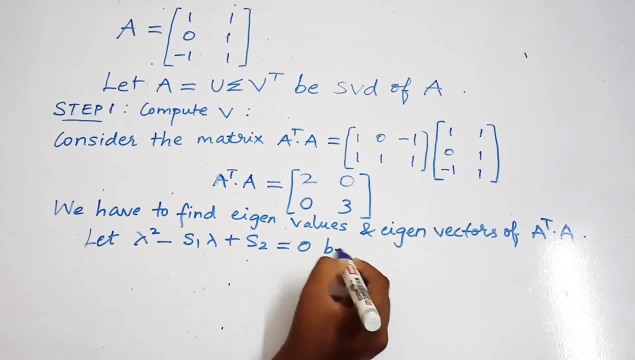 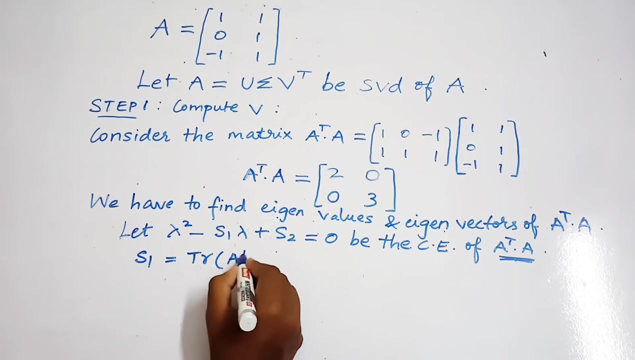 Plus S2 is equal to 0. Be the characteristic equation of the matrix A transpose A. Here S1 is trace of the matrix A transpose into A. So here trace is sum of diagonal elements. So 2 plus 3 that is 5.. Next, S2 is the determinant of the matrix A transpose A. 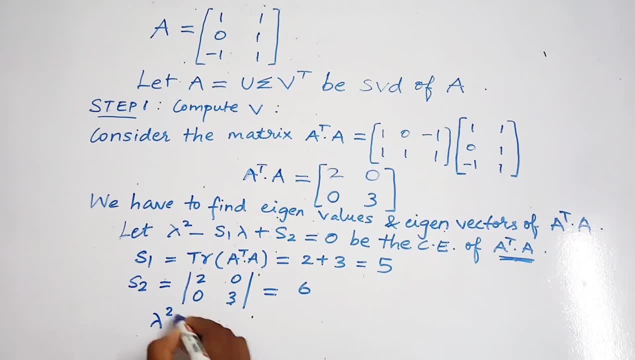 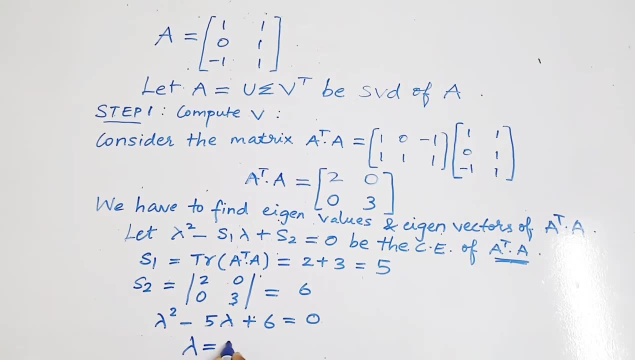 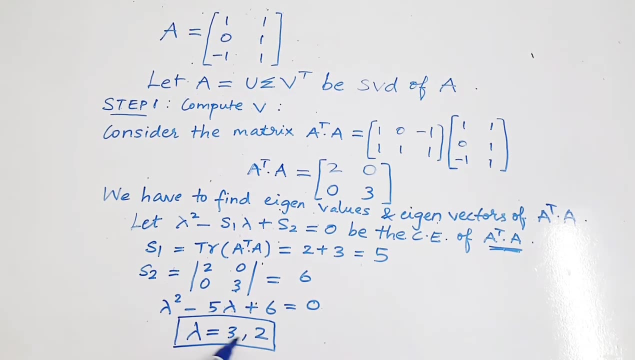 So here determinant value is 2, 3's are 6.. Now the characteristic equation obtained is lambda square minus 5. lambda plus 6 is equal to 0.. After solving this we will get: lambda is equal to 3 and 2.. So for SVD we have to write the eigenvalues in the decreasing. 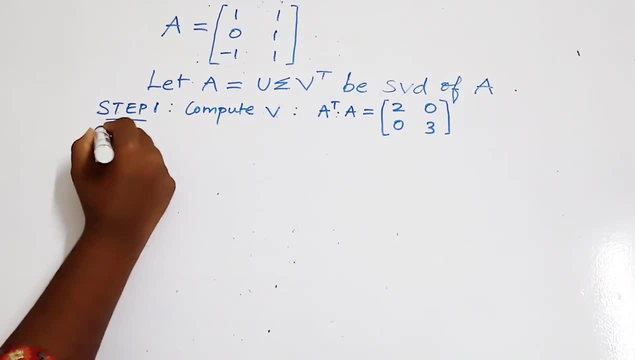 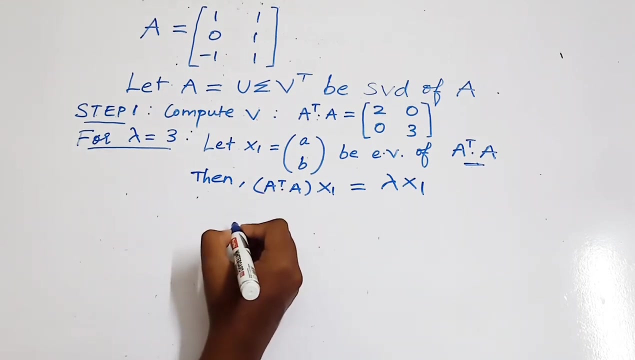 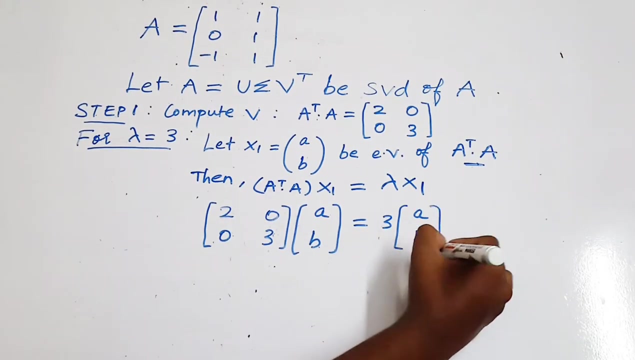 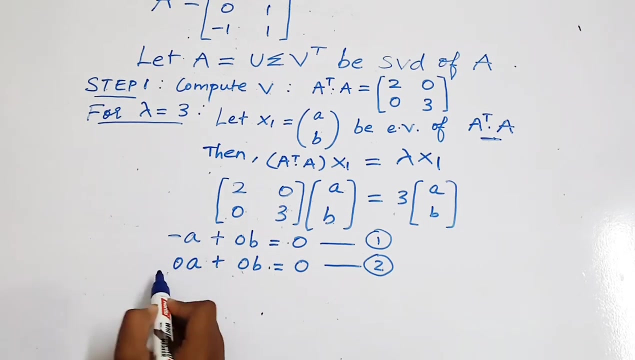 order. Next we will find the eigenvectors for the corresponding eigenvalues. Here I have taken X1 is equal to AB as the eigenvector. So then A transpose A, X1 must be equal to lambda X1.. We have obtained two equations after solving this. Since both equations 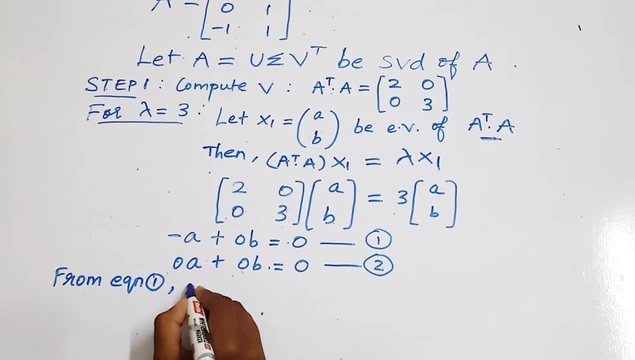 are same. consider equation number one and put random values for A and B And that should satisfy both the equations. So here I have taken A as 0 and B as 1. And the 0 and 1 are satisfying both the equations. 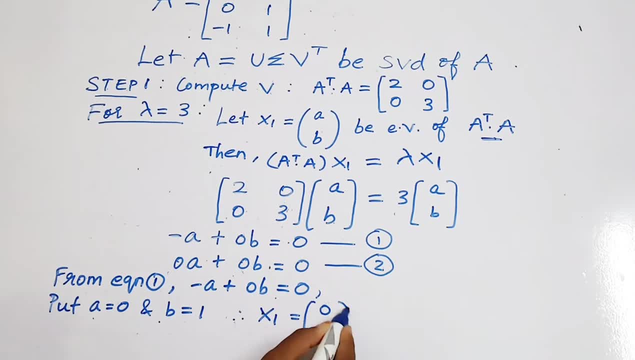 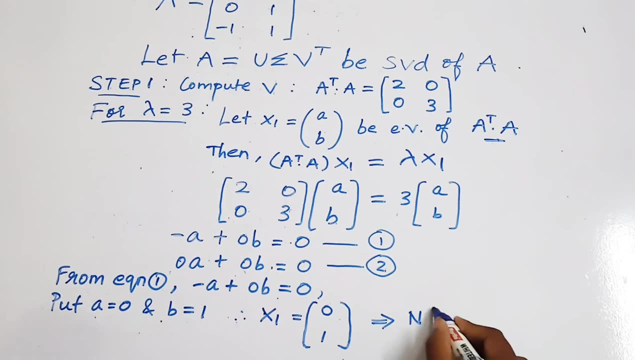 So the eigenvector obtained is 0, 1.. Next we have to normalise this eigenvector means divide each element of the matrix by its length. We have taught that. in what order? I have taught it before, Mainly the matrix understanding. 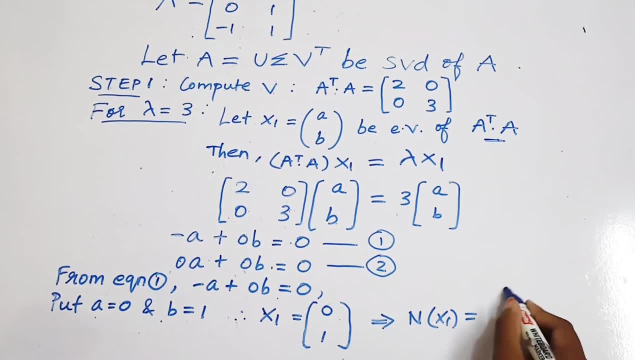 its length. here the length is one, so zero by one, one by one. so how do we find? the length means root of first element: zero square plus one square, that is one. so the normalized eigenvector is zero one. similarly i have found the eigenvector for lambda is equal to two. so we have found: 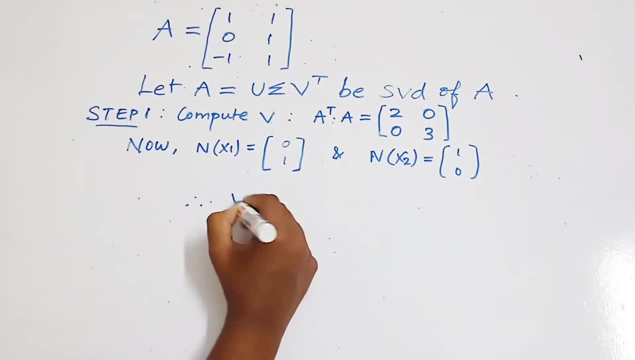 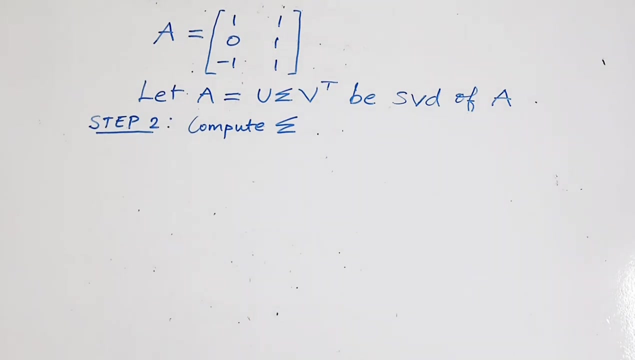 the normalized eigenvectors for the corresponding eigenvalues. so our v matrix is zero. one one zero. next we have to find v transpose. so v transpose is the same as v, as here v is a symmetric matrix. step two is computation of sigma matrix. here order of sigma must be equal. 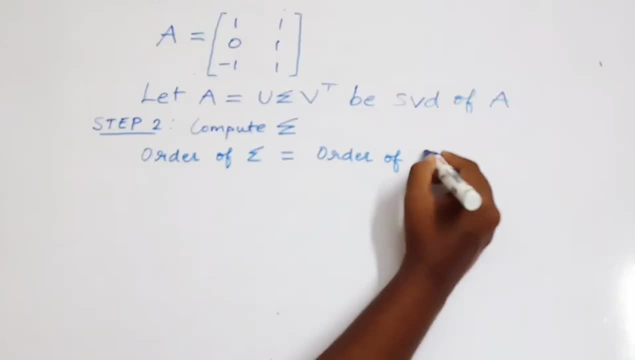 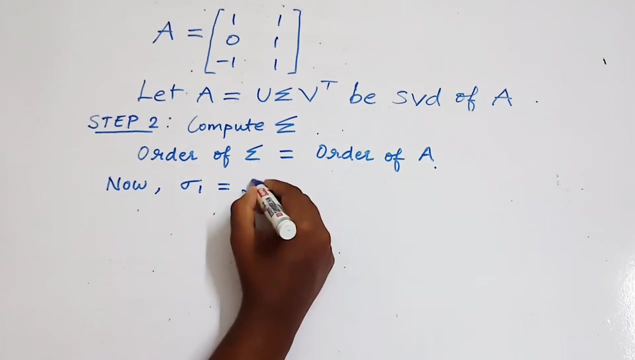 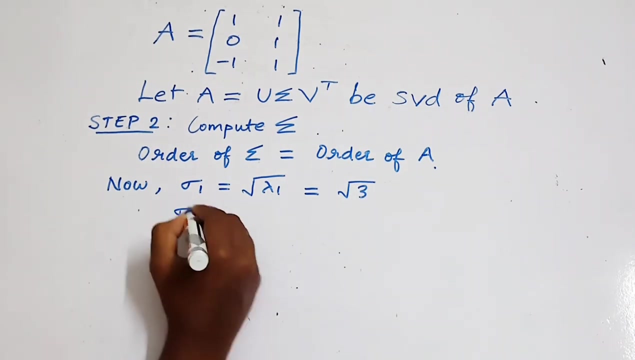 to order of a, That is, size of a and size of sigma should be the same. next we will find singular value, sigma one and sigma two. sigma one is equal to root of lambda one, that is root three. sigma two is equal to root of lambda two, that is root two. number of non-zero eigenvalues must: 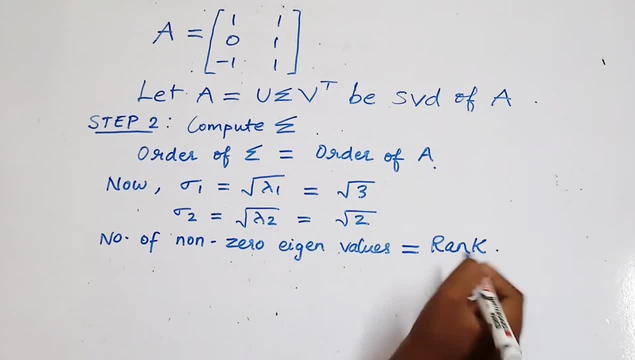 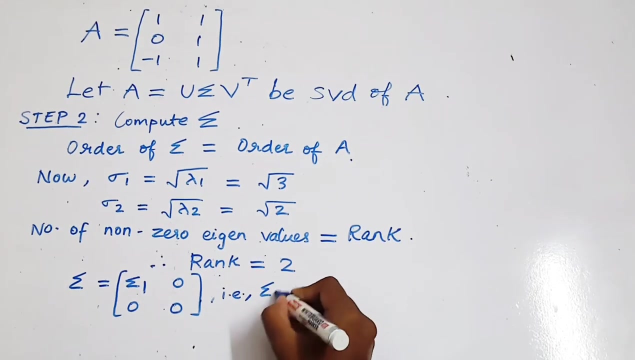 be equal to the three. Rank of the matrix. here number of non-zero eigenvalues are two. therefore rank is equal to two. next sigma matrix is written in this form, where sigma one is a diagonal matrix, whose Who is a Who is a Who is a matrix. so the 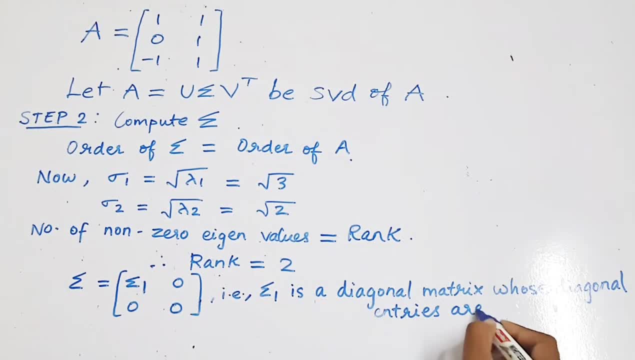 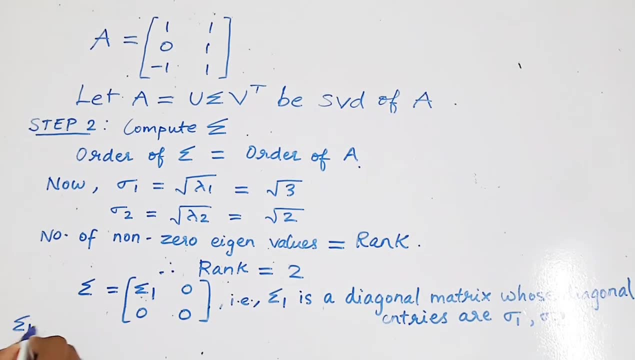 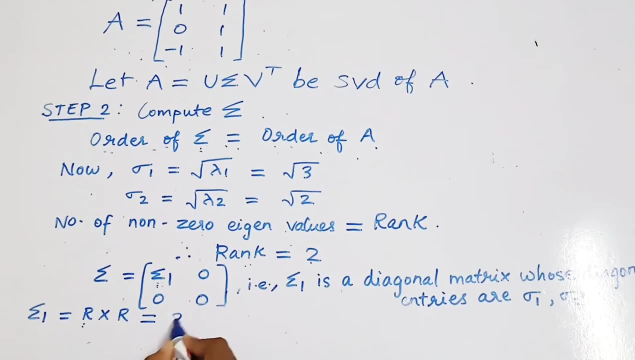 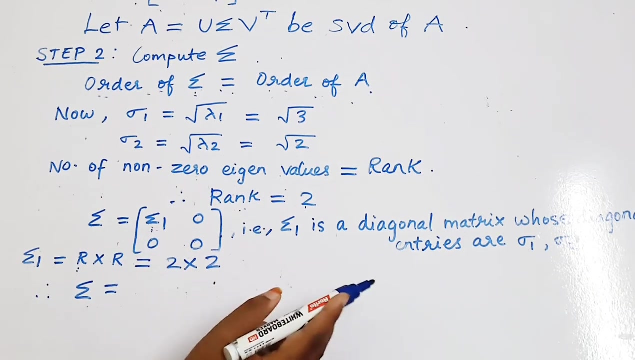 So the擊nolentries are sigma one and sigma two. order of the matrix. sigma one is r cross are. that is aerospace rank. so your rank is two. so two cross two. therefore the matrix sigma is equal to sigma one. sigma one is what diagonal matrix whose diagonal entries are? 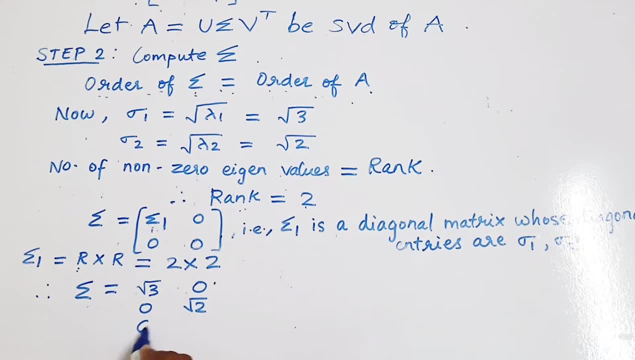 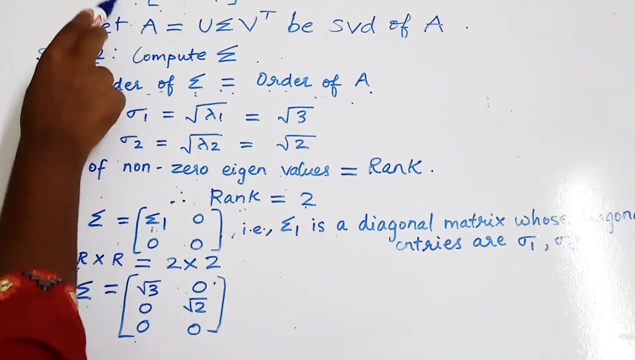 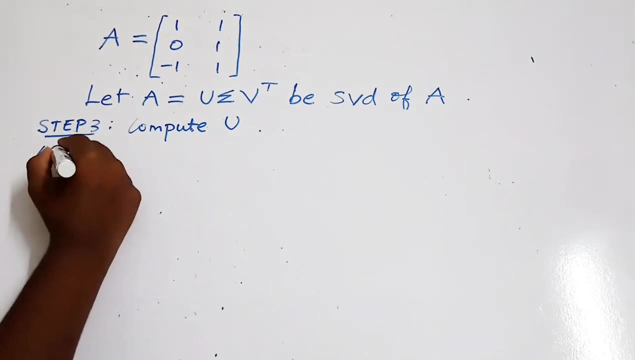 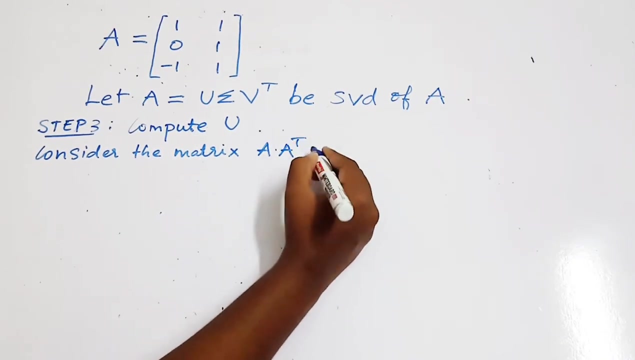 sigma one and sigma two. so root three: zero, zero. root two: zero zero. so why we are adding zero in the third row? because order of sigma should be equal to order of a. so this is a sigma matrix. step three is computation of matrix u. so for finding matrix u, consider the matrix a into a transpose. 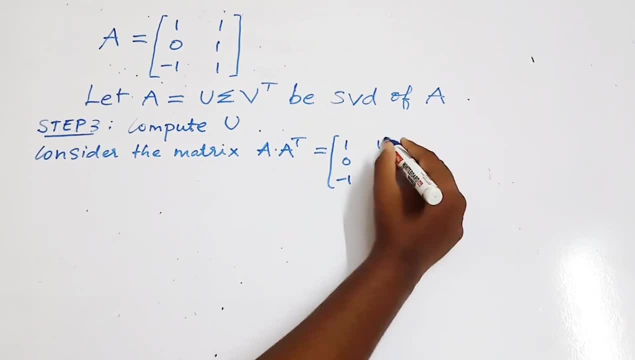 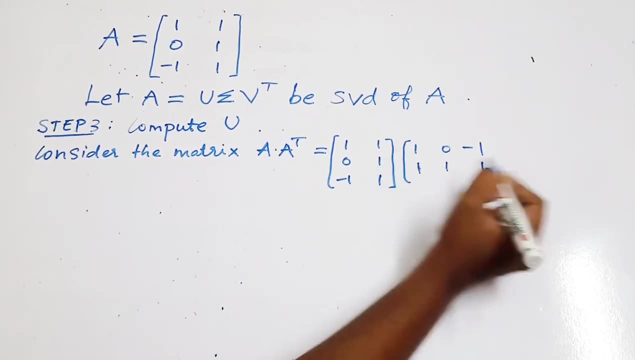 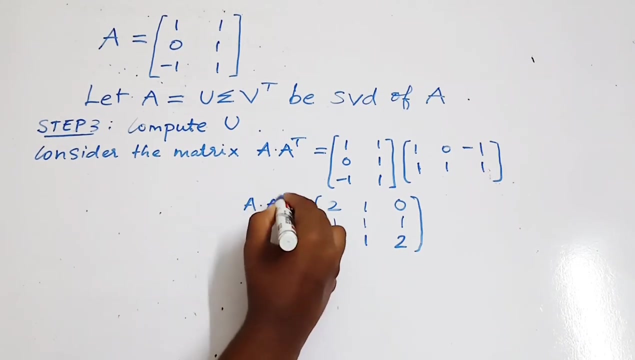 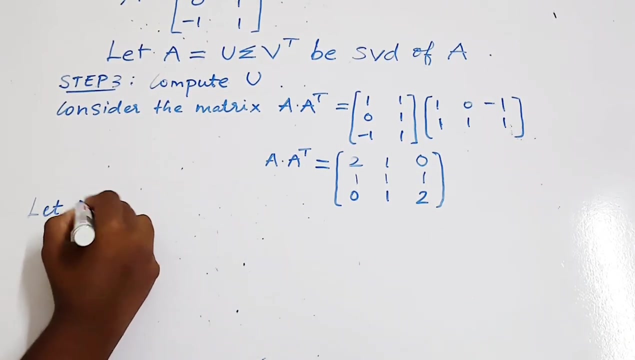 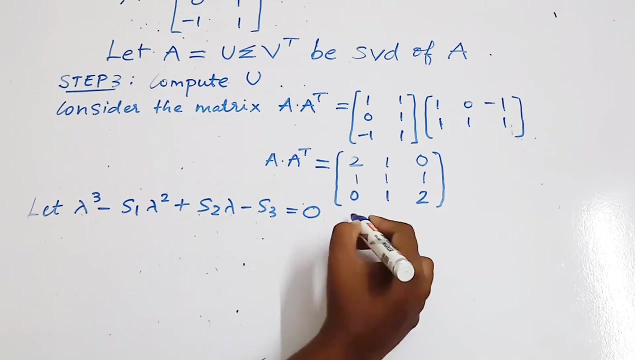 so we have to find the value of a into a transpose. next we will find eigenvalues and eigenvectors for this matrix. a a transpose, so we have to find the value of a into a transpose. let lambda cube minus s one, lambda square plus s two, lambda minus s three is equal to zero, be the characteristic equation of the matrix. 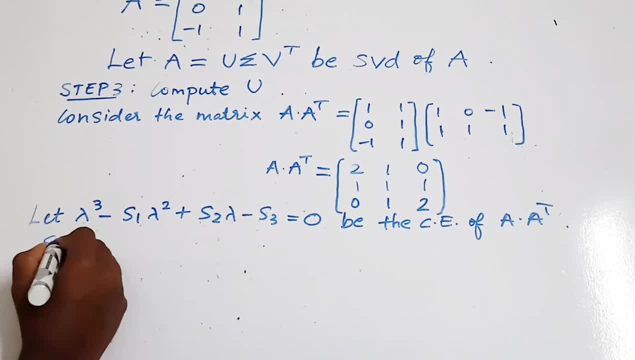 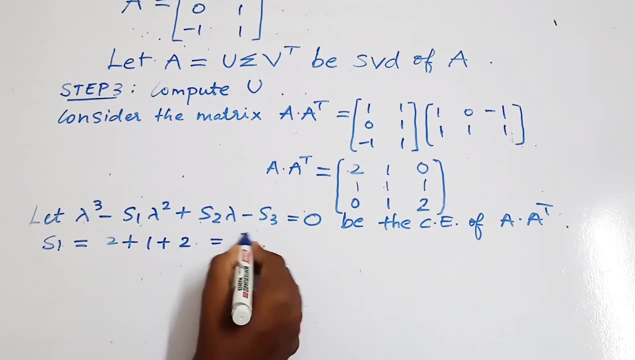 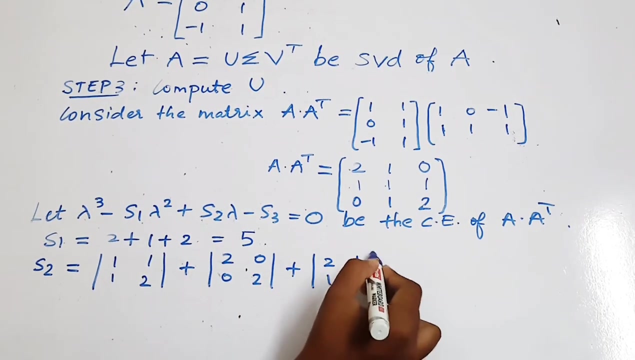 a a transpose. here s one is trace of the matrix a, a transpose. so trace is sum of diagonal elements. so two plus one plus two, that is five s two is sum of minors of the matrix a, a transpose. so we have to find the diagonal elements of the matrix a, a transpose value. 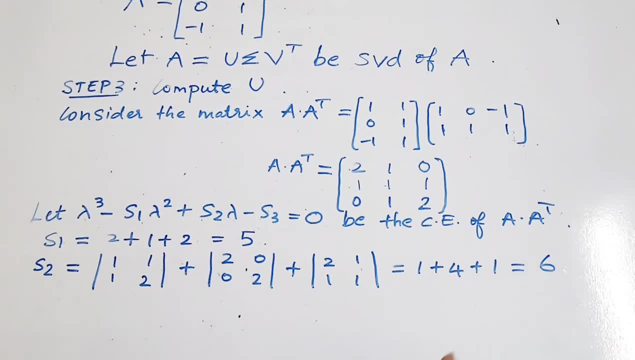 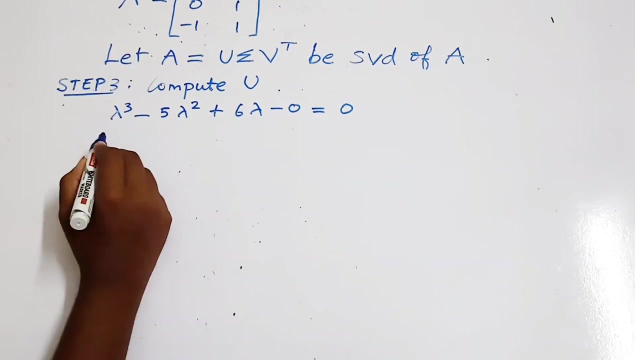 of s two is one plus four plus one, that is six. s three is determinant of the matrix a, a. transpose so two into one minus one into two, which is equal to zero. so the obtained characteristic equation is: lambda cube minus five, lambda square plus six lambda is equal to zero. we. 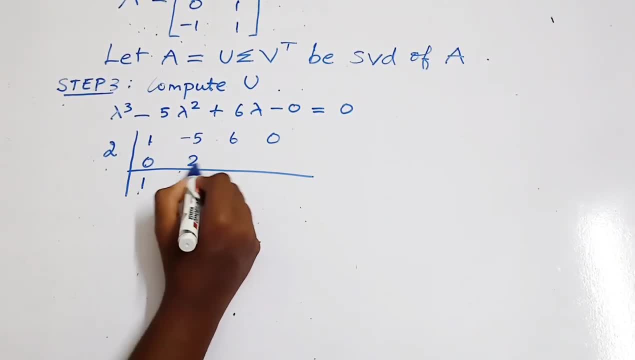 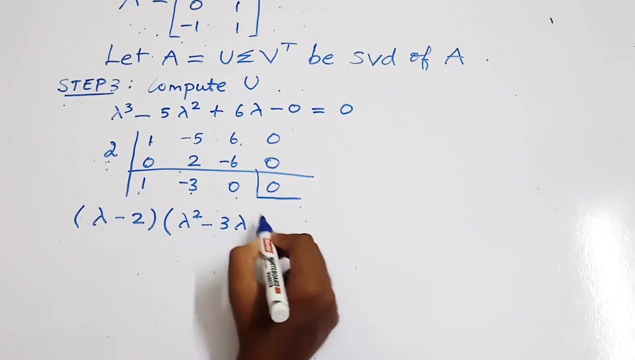 have to solve this cubic equation using factorization method. so here the factor is two plus four plus one plus one minus two. so we have to solve this cubic equation using factorization method. so the eigenvalues obtained are two zero three in s v d. we have to write those. 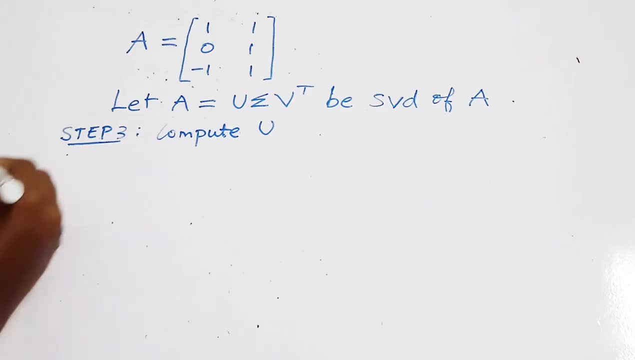 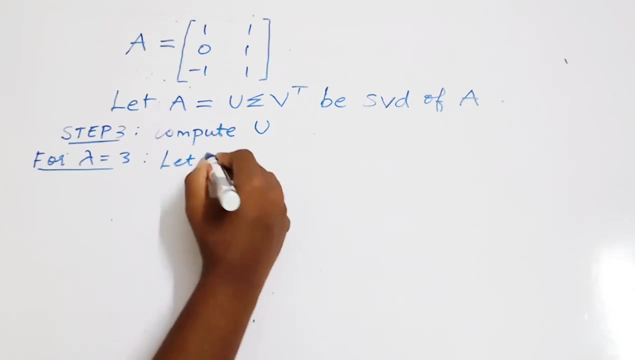 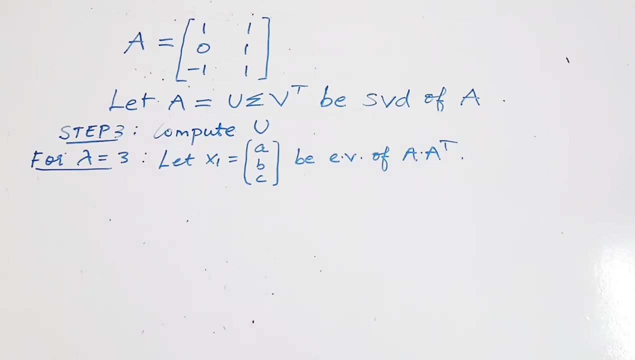 eigenvalues in the decreasing order and we have to write S, sl at x prime is equal to pi and we have to write the fraction. so we have to write the fraction at x prime is equal to. Next, we have to find eigenvectors for the corresponding eigenvalues. 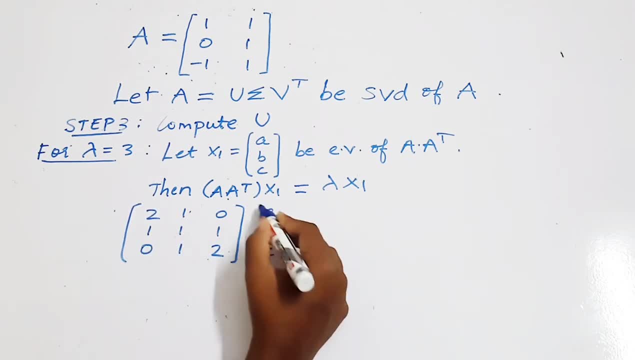 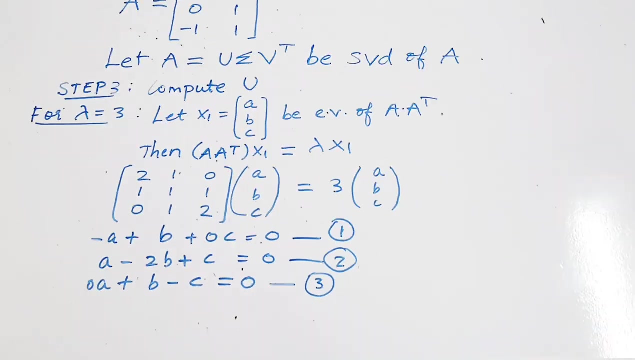 We have to solve these three equations. We have to solve these three equations. Consider the first two equations. Consider the first two equations: First write the coefficients of B, Then coefficients of C, Then coefficients of A, And then again write the coefficients of B. 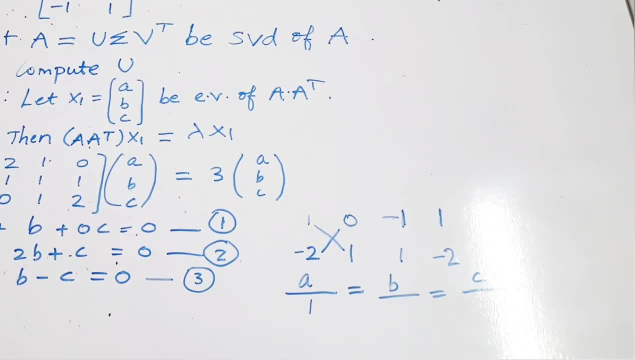 Next we have to cross multiply. So A by 1 is equal to B by 1 is equal to C by 1.. The values of A, B, C are 1, 1, 1.. Therefore, x1 is equal to 1, 1, 1.. 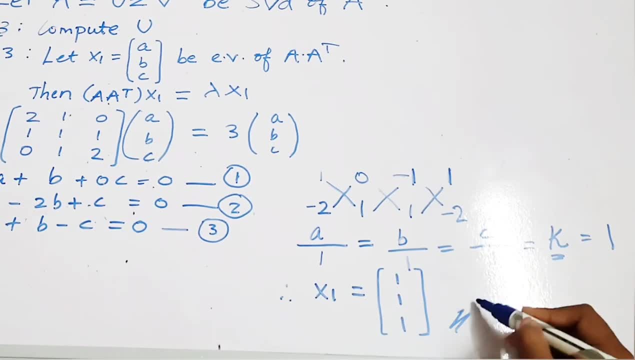 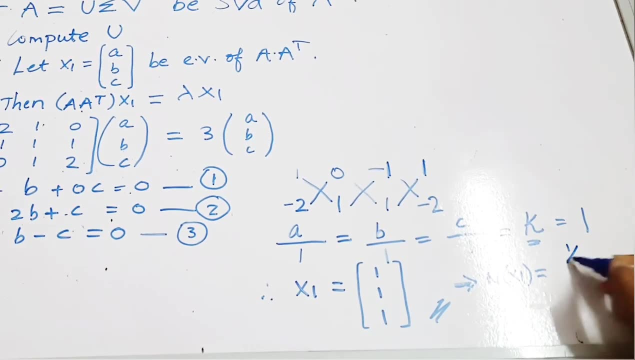 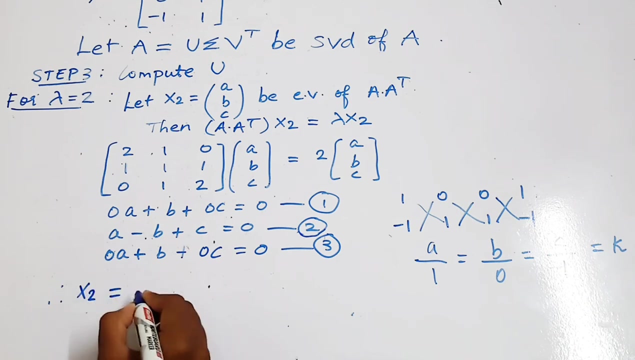 Next we have to normalize this eigenvector, So n of x1 is equal to 1 by root 3, 1 by root 3, 1 by root 3.. Similarly, the other two normalized eigenvectors for the corresponding eigenvalues: